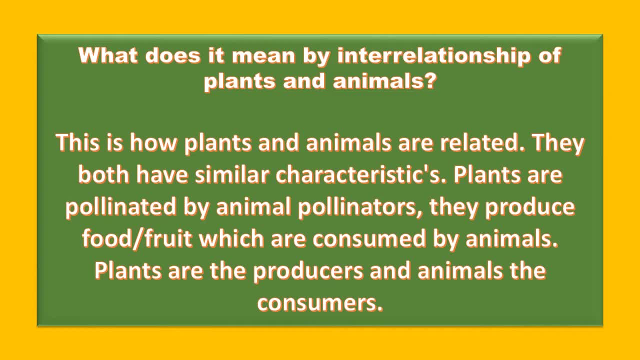 and animals are related. They have similar characteristics. In order for plants to be pollinated, the pollination has to be done by other animals or animal pollinators, such as bees. They produce food, such as different kinds of fruits, and all those different kinds of fruits are then consumed by animals, for example humans. 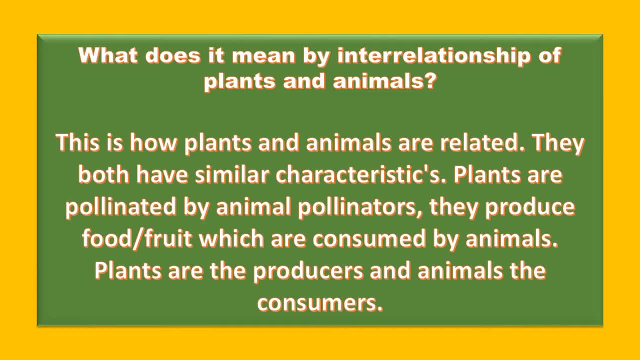 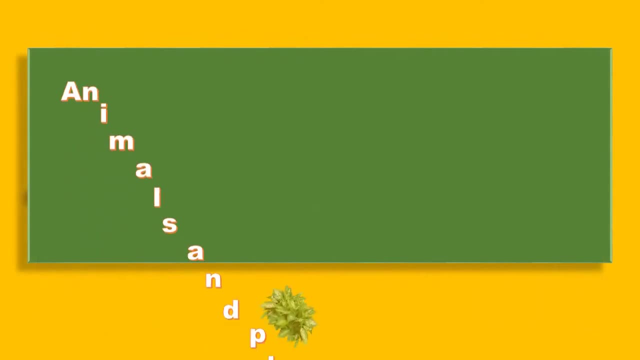 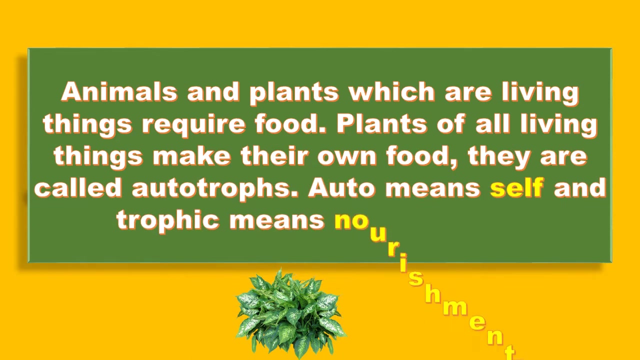 Now we know that plants are producers- They produce the food, And animals are the consumers. What the plants produce, the animals consume, such as us humans. Animals and plants, which are living things, require food, All living things require food. Plants, of all living things, makes their own food. Therefore, 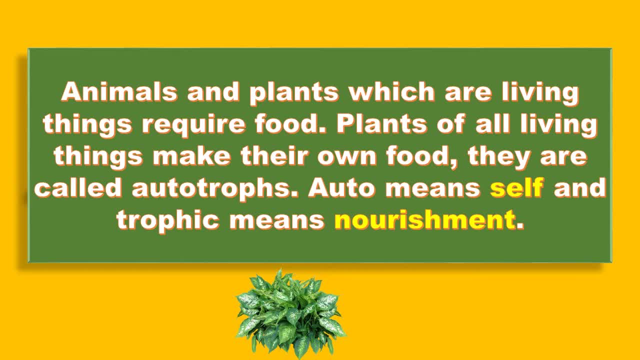 they are called autotropes. Now, the reason they are called autotropes is because they are able to make their own food. Auto in the word autotropes means self And tropic means nourishment. Together you get the word autotrope. 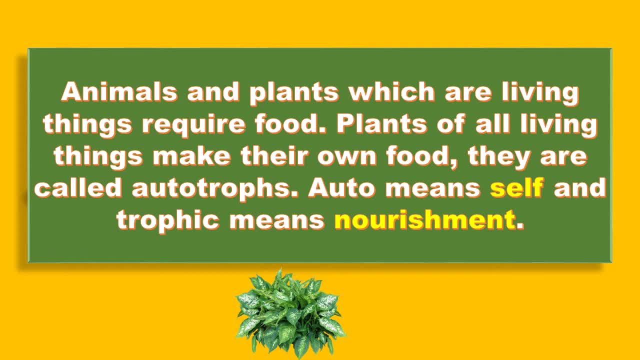 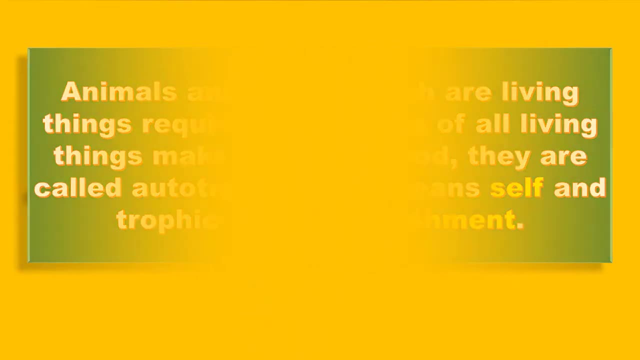 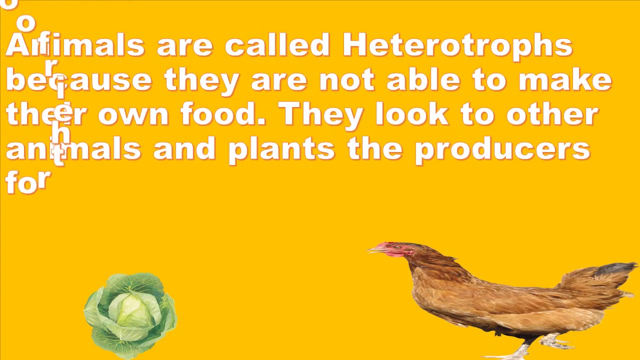 So that shows that plants, of all living things, are able to make their own food. They have that ability, the word given That ability to be able to make their own food, While plants are able to eat their own food right, Because they are given that ability. 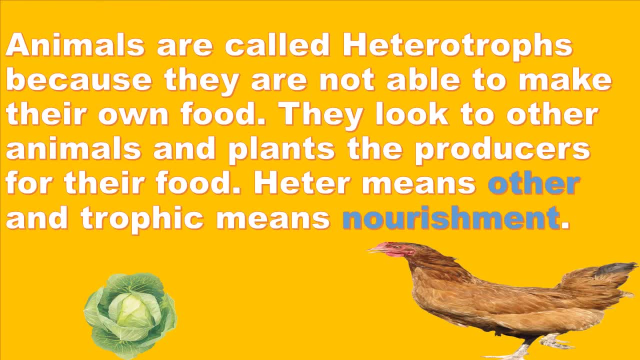 Animals are not able to make their own food, so therefore they are called heterotrophs. They have to see food from other animals and plants whom other produces for their food. Other in the word, heterotroph means other and trophic means nourishment. 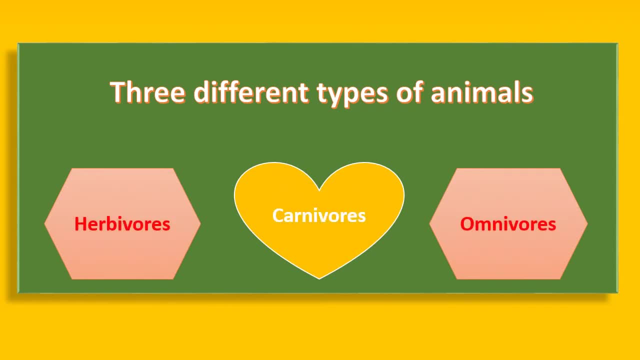 Now we're going to look at the three different types of animals, The three different types of feeders that exist in society. There are three different types, and we have herbivores- There are others- And birds- There are other animals, There are many other animals. 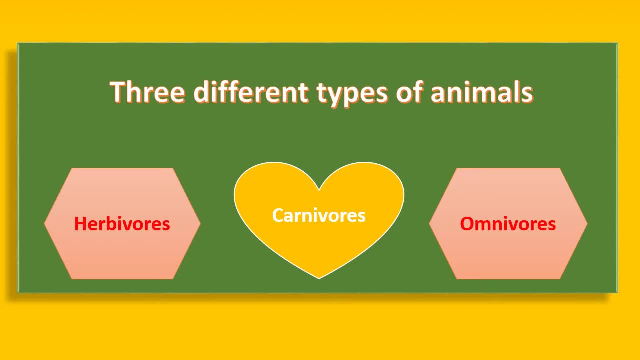 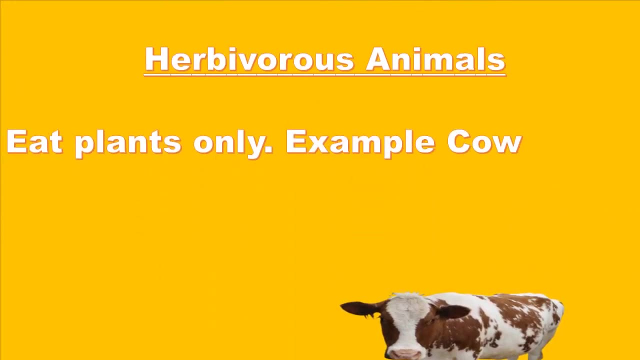 carnivores and omnivores. so now we're gonna look at each feeder. first one we have is herbivores- animals which are herbivores. now, herbivores are herbivores animals. they are plant eaters only. they only consume plants. for example, we have the cow. 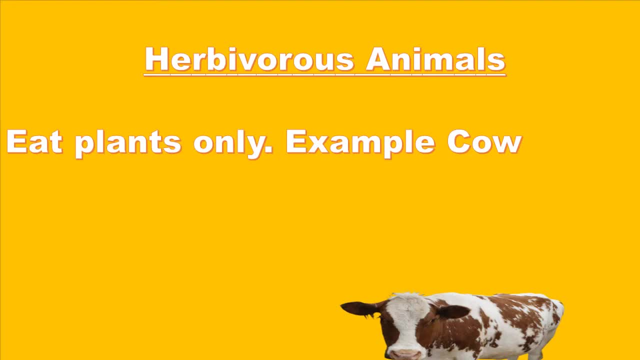 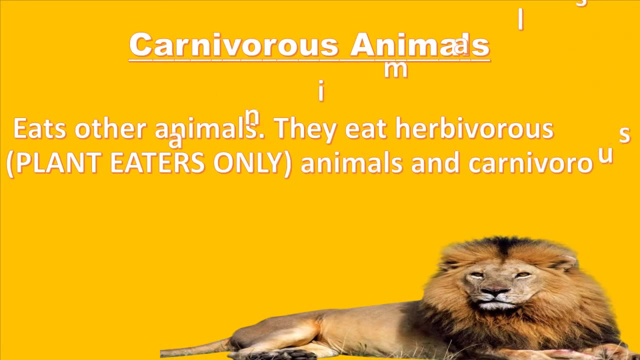 and we know that the cow consumes grass. now we're looking at carnivores animals, which are known as carnivores. there are two different kinds of carnivores animals. you have the first set, who eat other animals, who only consume plants. then you have the other animals whom they eat. 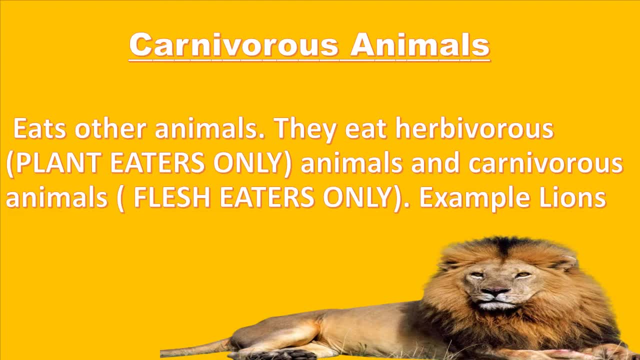 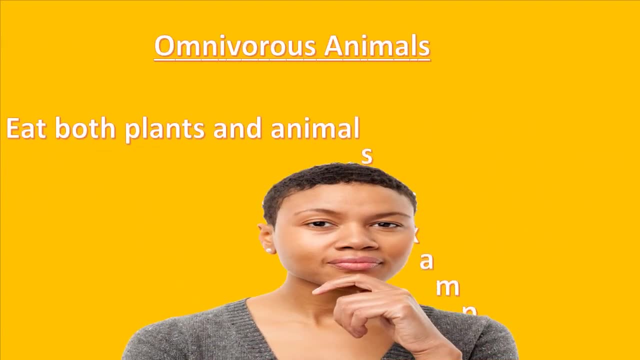 that only eat flesh, wool. now we're looking at omnivores- animals. omnivores- animals- are known as omnivores, which e plants and animals. so, for example, as you can see the lady on the screen, she is a human and she consume both plants and animals. so, for example, we eat cabbage. a. 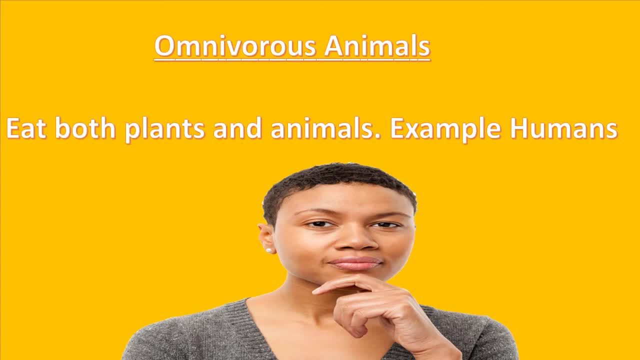 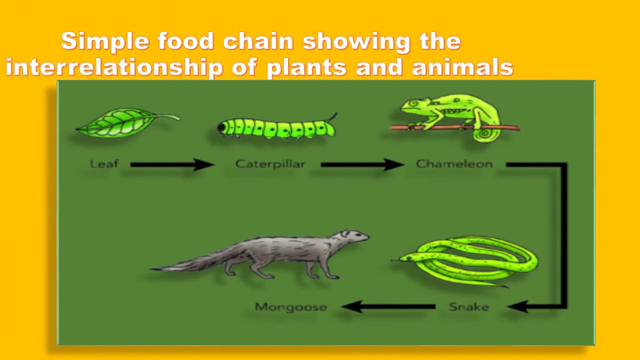 plant and we also eat chicken or we eat fish, which is a animal. so omnivorous animals eat both plants and animals. simple full chain showing the interrelationship of plants and animals. now, what starts off the food chain? the whole chain starts off with the leaf. What is the leaf? the leaf is known to be the producer, whose the producer again. 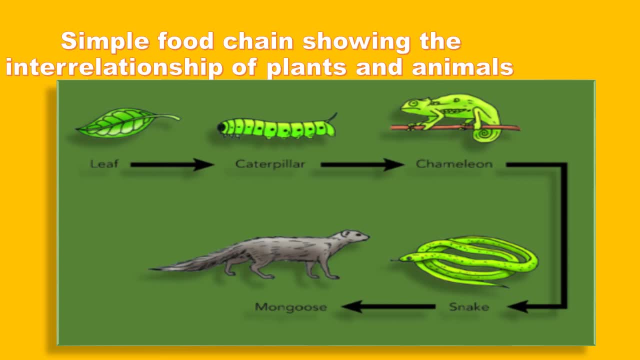 the producer are known to be plants because they are able to make their own food. Now the leaf. there is the producer and it starts the food chain. Now who will consume the leaf? The leaf will be consumed by the caterpillar. Who is the caterpillar? The?